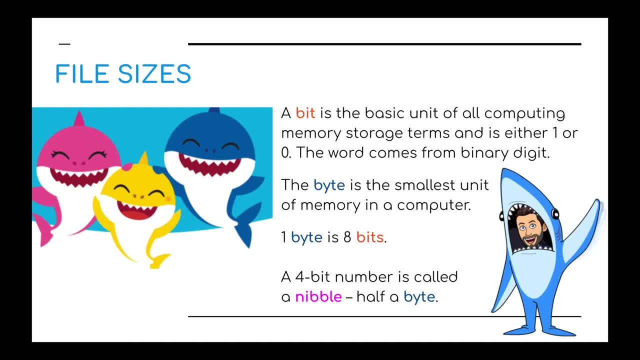 are called a byte. The byte is the smallest unit of memory in a computer. One byte, of course, equals 8 bits And the one in between, Mummy Shark, is halfway between a bit and a byte, and this is four bits of information, and this would 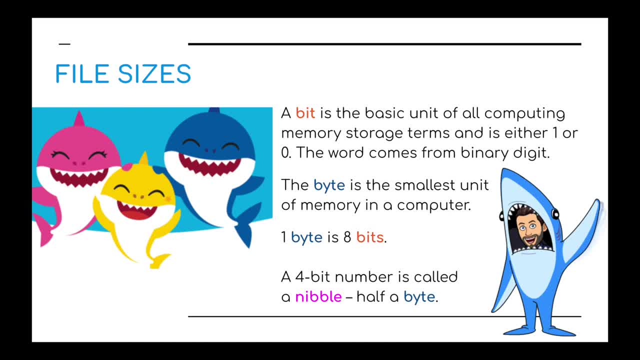 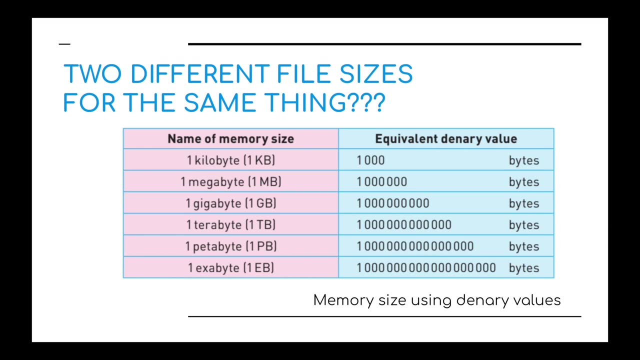 be considered to be or called a nibble. So we've got a bit Baby Shark, we've got a nibble Mummy Shark and we've got a byte Daddy Shark. Now we can look at file sizes in two different ways: The 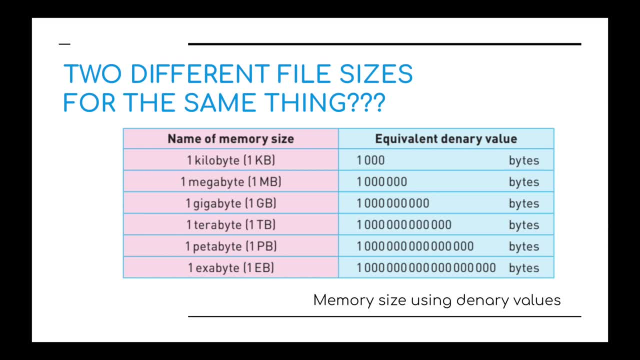 first method we use the used denary values. so for example, a kilobyte would equal a thousand bytes, 1 KB. We multiply that by a thousand and we get one megabyte. Multiply it again by a thousand a gigabyte. 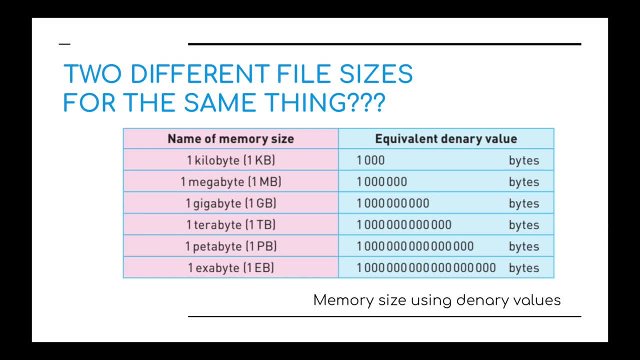 and we go up in thousands every time. So from a gigabyte to a terabyte, to a petabyte, to an exabyte, As you can see, each time we've added three zeros on the end of each one to get the relevant value. So we're dealing with lots, and 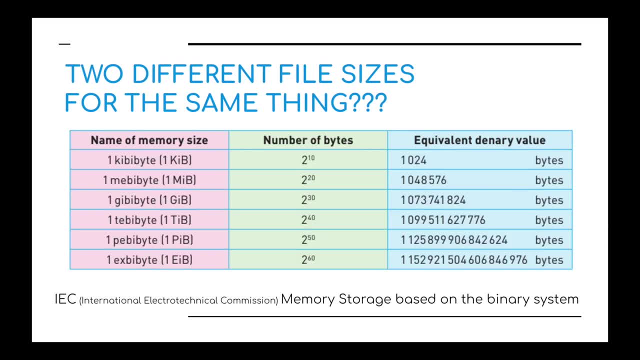 lots and lots and lots of zeros. Now, the other way, we're going to the power of two, to the power. So, for example, in the book and this- I've never seen this before, but this is interesting- this is the IEC, the International Electro-Technical Commission- memory. 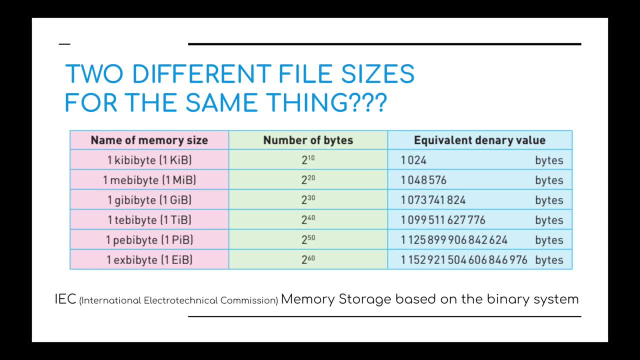 storage method based on the binary system. So let's say 2 to the power 10,, 2 to the power 20, and so on and so forth. But we've changed the name, it's no longer a kilobyte. I. 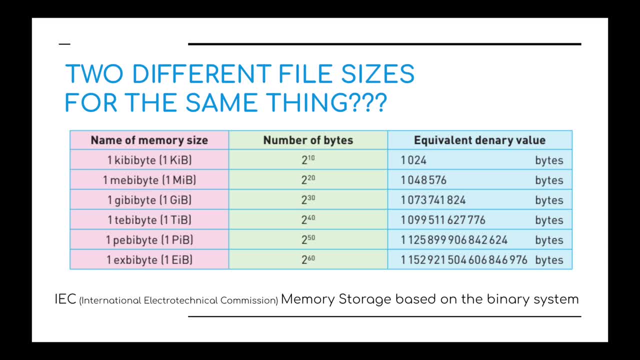 don't know whether this is for the benefit of IGCSE or what, but we're going. we're basing this on Kibibytes, So one Kibibyte is 2 to the power 10, so 2 times 2 times 2. 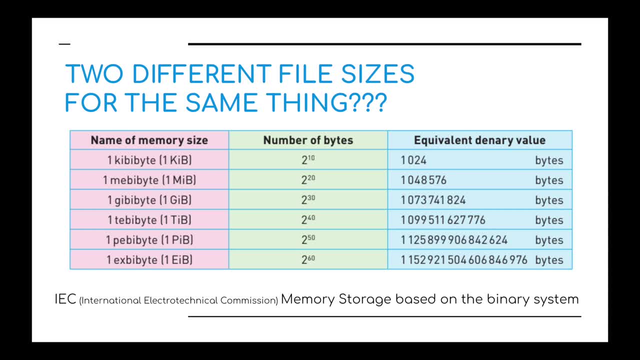 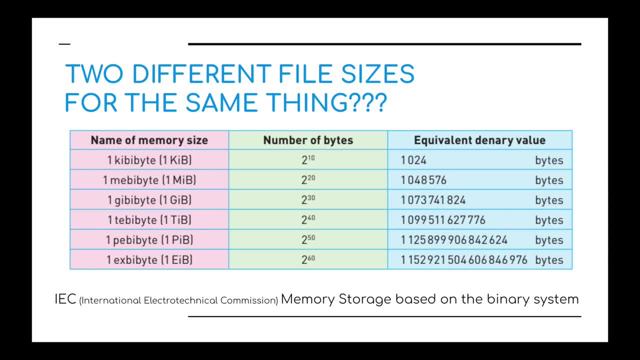 going up each time. So right up to an exabyte, which would be 2 to the power 60. As you can see, there we've got a lot of a very, very, very big number. So that's the two different methods Now, the old way, when you were showing out your working. 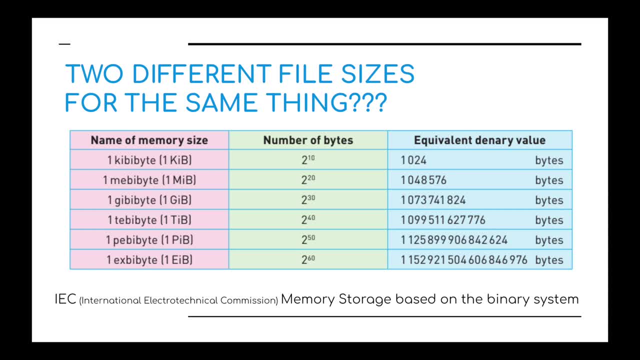 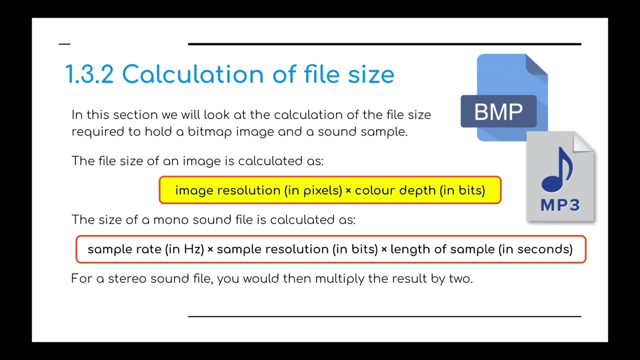 out when you were doing calculations. based on this, you could do it. either way, I'm not sure what the exam board are expecting now. we'll have to wait and see and watch this space on that. So now that we know about the different file sizes, 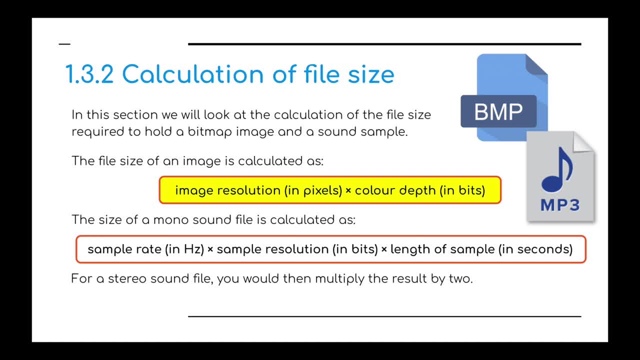 and be that going up in kilobytes or Kibibytes. we need to be able to establish how we can do calculations on bitmap images and on sound samples, some sound files. So in the first instance, we're going to look at calculating the size of an image, and this is based on the image. 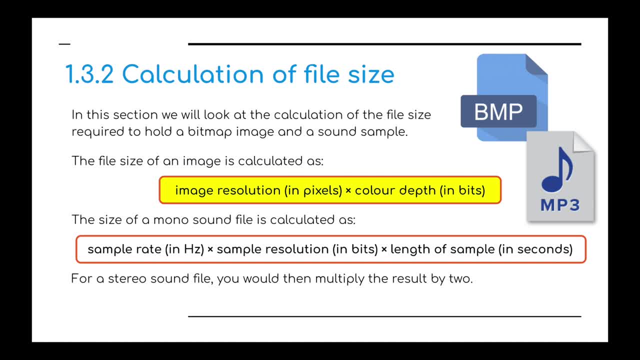 resolution, ie the number of pixels. the image has the pixel matrix, which I'll come onto in a moment, and we multiply that by the color depth in bits. For a sound file- and this is for a mono sound file- we use the sample rate, the number in Hertz, and we multiply that. 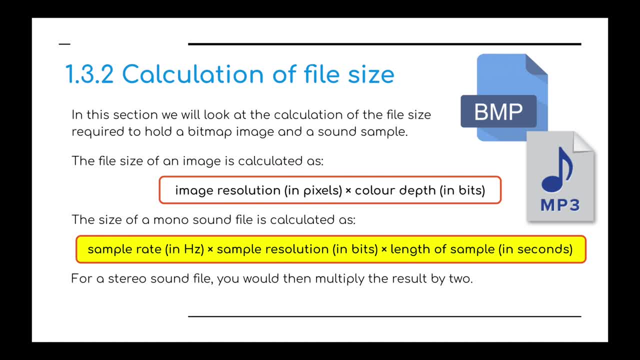 by the sample resolution, which is measured in bits, and then we times that by the length of the sample, which of course is measured in seconds. how long it will be If we want to turn this into stereo sound, which generally we would do. 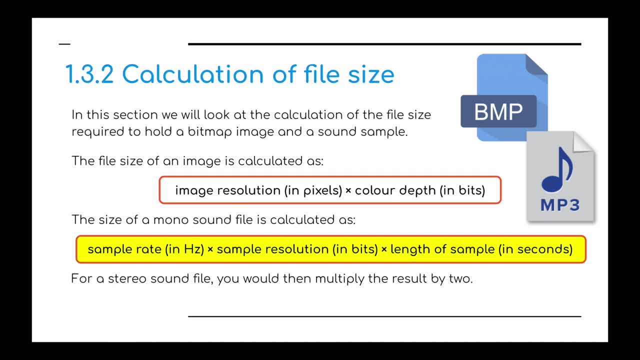 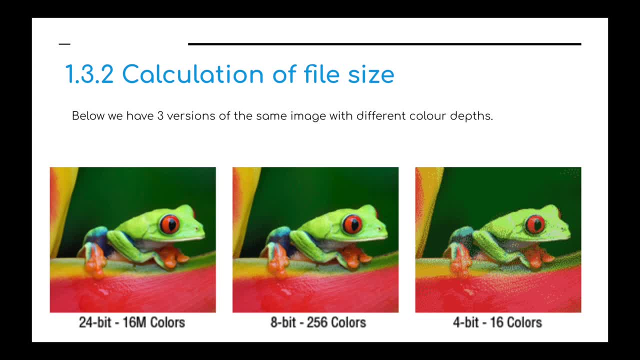 we will multiply the entire thing by two. So I have an example here, three pictures of a tree frog: one in 24-bit, 16 million colors, 8-bit, 256 colors and finally a 4-bit, which would give us 16. 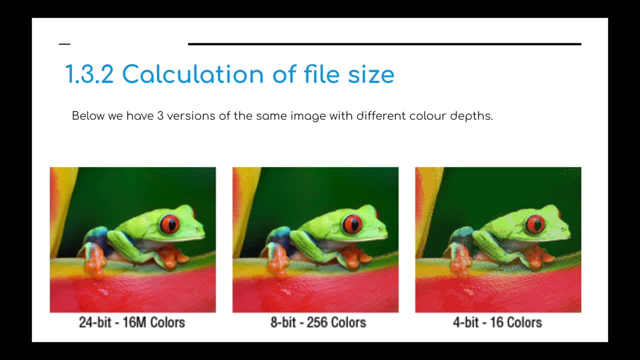 colors, So three different versions of the same image. Now, if we were to guesstimate that this image was 250 by 300 pixels in dimensions, that would give us a total pixel matrix. so multiply on the x-axis by the y-axis. 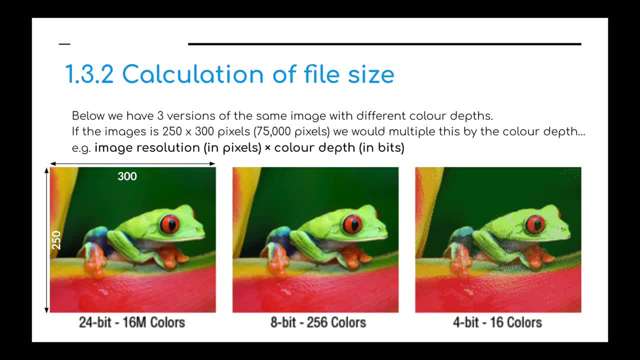 by 75,000 pixels. okay, We then would multiply that by the color depth. so if we were to say it was multiplied by 24 bits, we would get a value of 1.8 million bits. If we were to times each of those, we would get a value of 1.8 million bits. 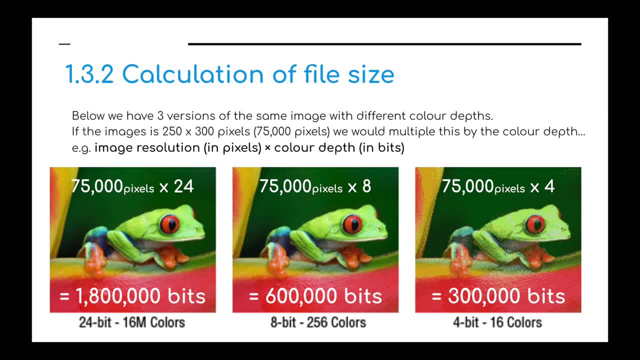 Times it by 8, 256 colors, we would get 600,000 bits. and then, if we multiply it by 4,- 75,000, multiplied by 4,, we would get 300,000 bits To work that into. 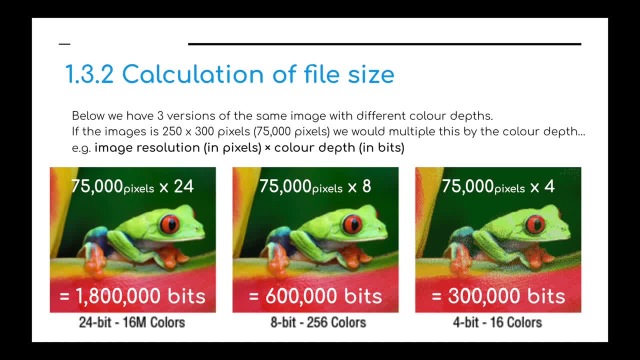 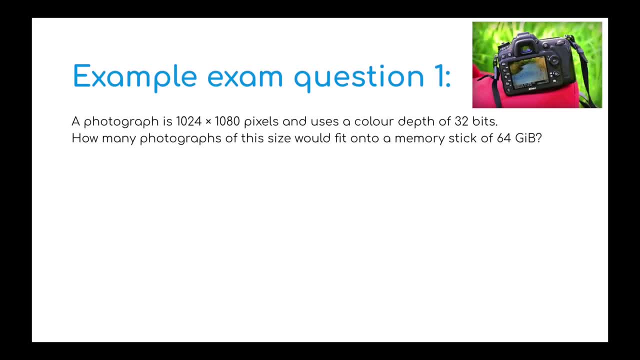 bytes. we would divide that number by 8, because of course there are 8 bits in one byte. For the last part of this video, I want to go through a few exam questions which might crop up on your exam. So first of all, we're going to look at measuring the size of an image. So exam: 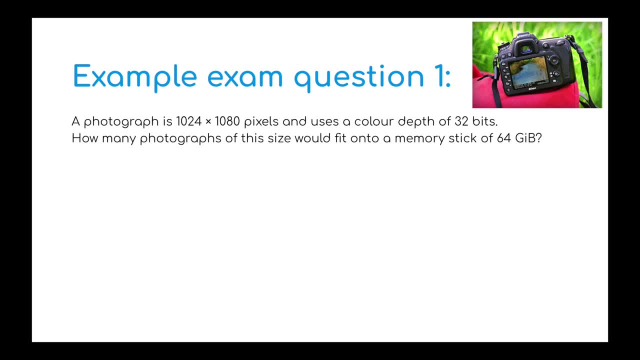 question 1,. a photograph is 1024 by 1080 pixels and it uses a color depth of 32 bits. How many photographs of this size would fit onto a memory stick of 64 gigabytes? Okay, we've put the i in between, so it must be gigabytes. 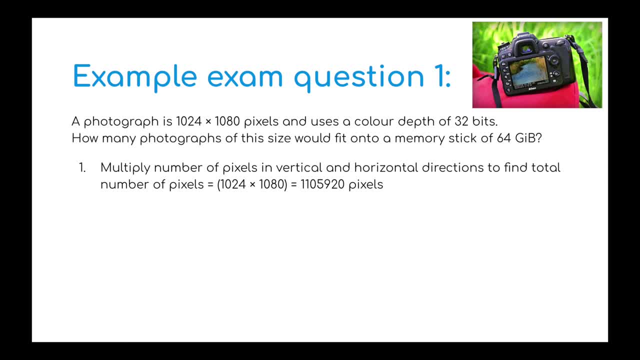 So first of all, job number one, we multiply the number of pixels in vertical and horizontal directions, x and y axis, to find the total number of pixels. So that would give us a number of 1105920 pixels. We then multiply the number of pixels by the color depth and then divide by 8 to give. 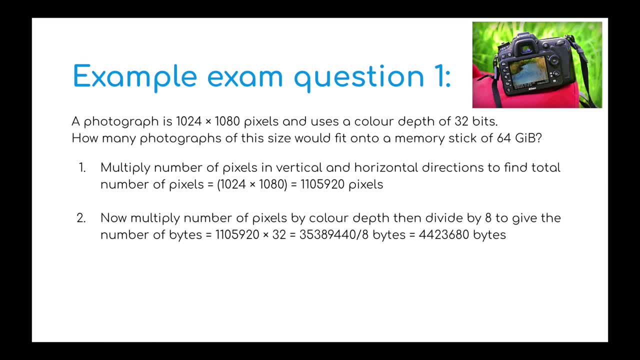 the total number of bytes. So 1,105,920 multiplied by 32, gives us that number there. Divide that by 8, would give us a total of 4,423,680 total bytes. To calculate how it would go onto a 64-gigabyte drive, we first of all take 64,. 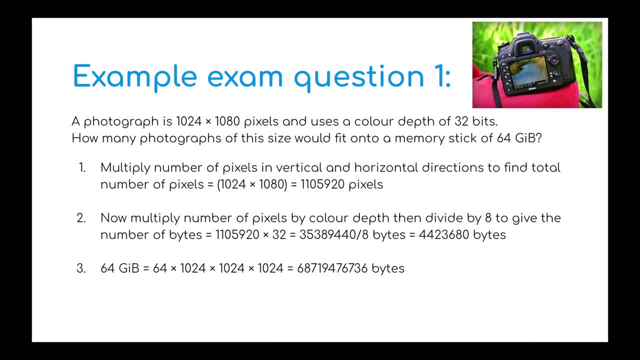 and we multiply it by 1,024, which would give us going into bytes, to kilobytes. multiply again by 1,024,, which would give us megabytes. multiply again by 1,024,, which would give us the gibibyte example. So that would be again. 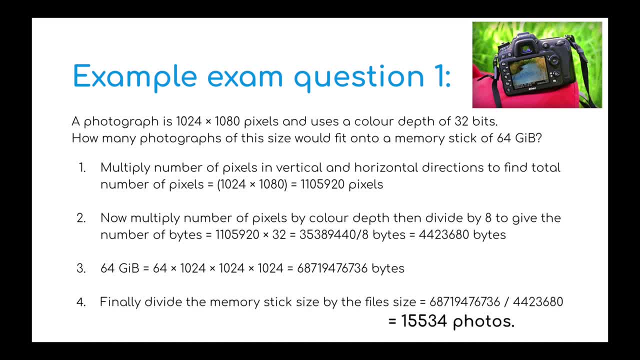 another massive number starting with 6,, 8,, 7 bytes. So finally we take that number and we divide. so finally we divide the memory stick size by the file size. So we take that original number, divide it by 44,. 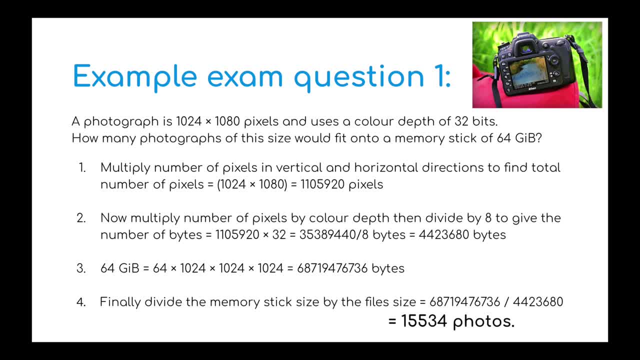 4,423,680, and we can see we can store 15,534 photographs. Lots and lots of big numbers. Now, one thing that students always ask, and I do not know whether this will be the case, or even whether these sort of questions, albeit these, are: 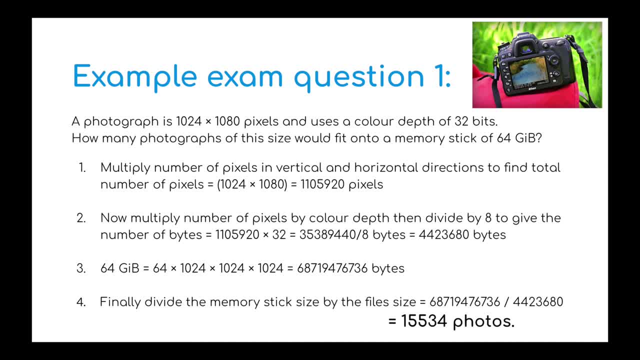 example, past paper questions will be on the paper, because it does say that the students are not allowed to use a calculator on either paper 1 or paper 2. now, So I don't know what's going to happen there, but that is basically how. 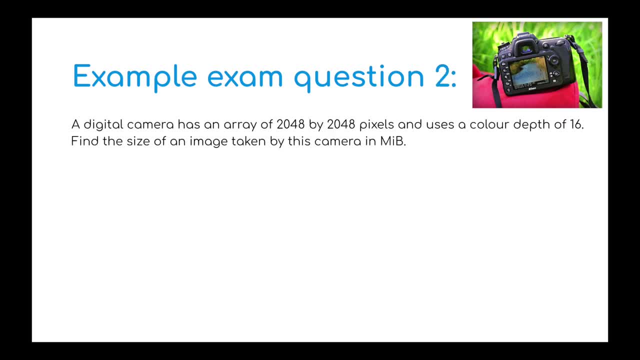 you would calculate. Now the second example, probably slightly easier, exam question 2,. we have a digital camera and it has an array of 2048 by 2048 pixels. Basically, the x-axis is 2048 pixels, So it's the y-axis, the grid matrix, and uses a color depth of 16, so 16-bit color. 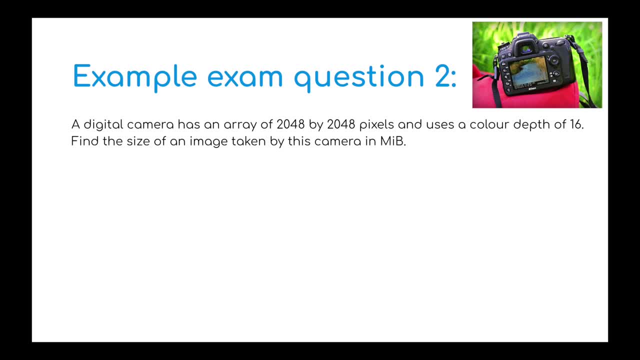 depth. Find the size of an image taken by this camera in mibibyes. Multiply number of pixels in vertical and horizontal directions to find out the total number of pixels. Well, there we go. we've got 4,194,304 pixels Now. 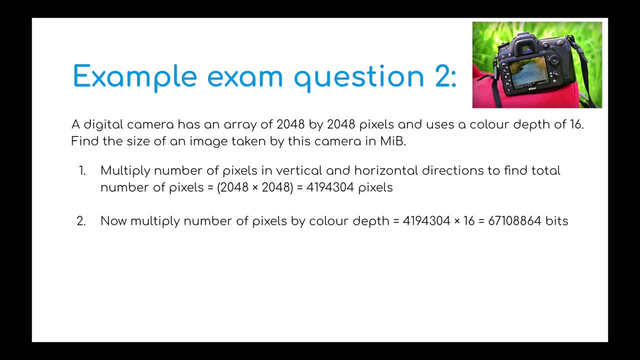 multiply the number of pixels by the color depth. so we're timesing that by 16.. So it's 67 million just over. Now we divide the number of bits- 67 million bits. we divide that by 8 to get the number of bytes. So there we go, we've got 8,388,608. 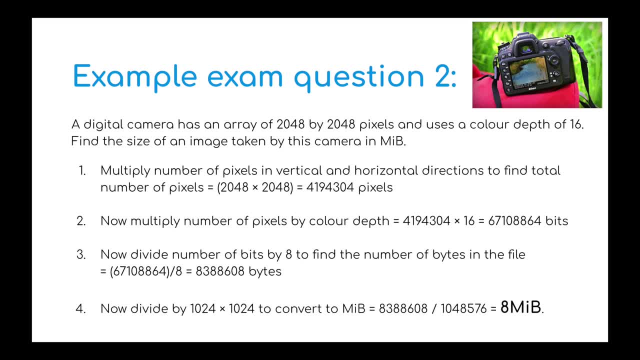 bytes. And then, finally, we need to convert the number of bytes. we have the 83.8 million and we need to convert those bytes into mibibytes. So, if you remember from last time, we're moving up in thousands. so we go from: 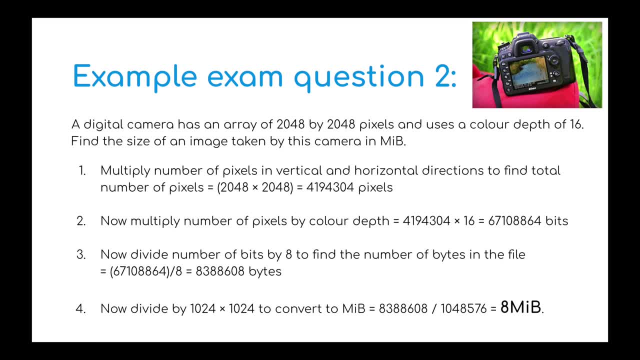 bytes to kilobytes to megabytes. So to do this we need to multiply 1024 by 1024 to give us a total of 1, just over 1024, so that's over 1 million 1,048,578.. And we're going to divide our original total, our number of 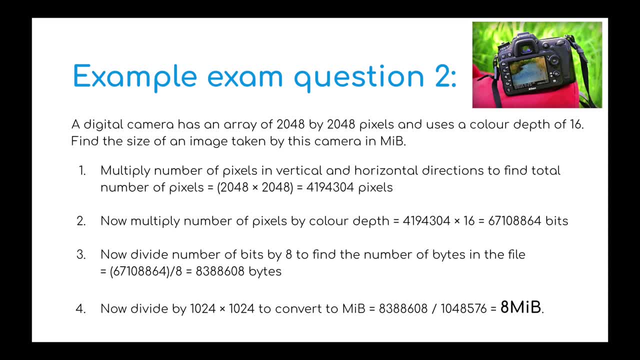 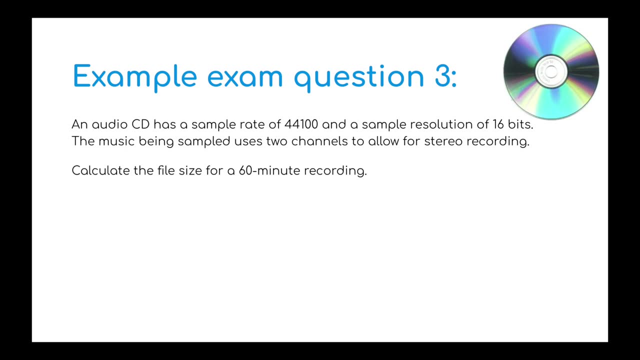 bytes by that figure, so 83.8 million divided by just over a million, and we will end up with a final total of 8 mibibytes. Now for the final, one final question. I'm going to move on to sound. So we've got an. 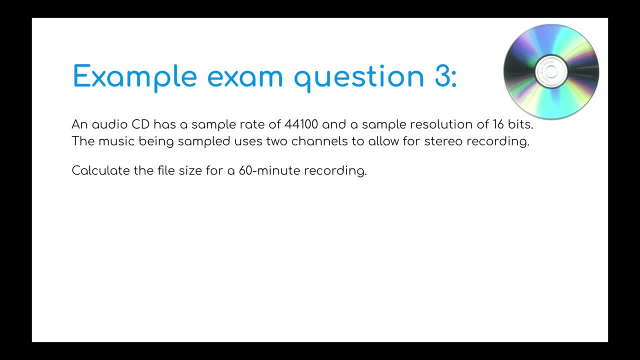 audio CD. Again, these don't really exist anymore, but it's how we used to store them, how we used to buy songs, buy music back in the day. So we have an audio CD and it has a sample rate of 44,100, and a sample resolution of. 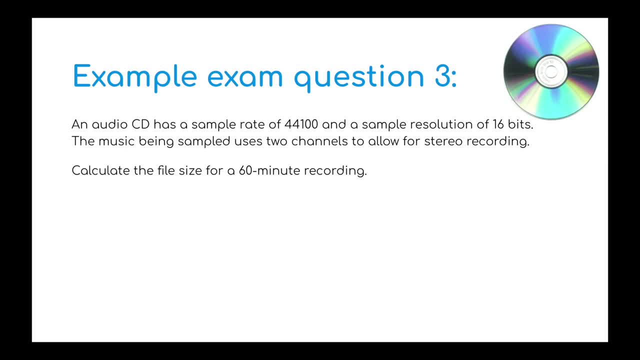 16 bits. That's for the ambulance to go past. The music being sampled uses two channels: stereo, to allow for stereo recording. Calculate the file size for a 60-minute recording: Okay, So 60 minutes of music going onto that CD. 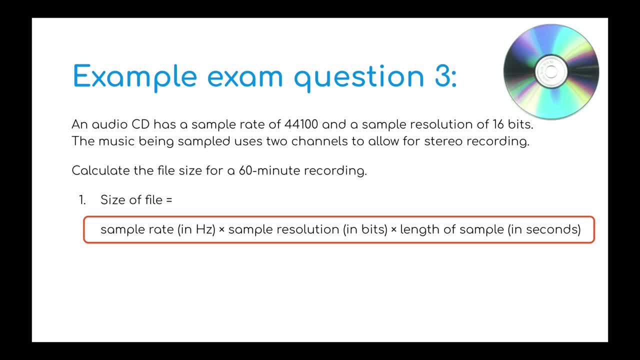 So the size of the file- remember the calculation from before- the sample rate in hertz times the sample resolution in bits, times the length of the sample in seconds. So we've got the value in hertz 44,100, we've got 16 bits for the sample resolution and. 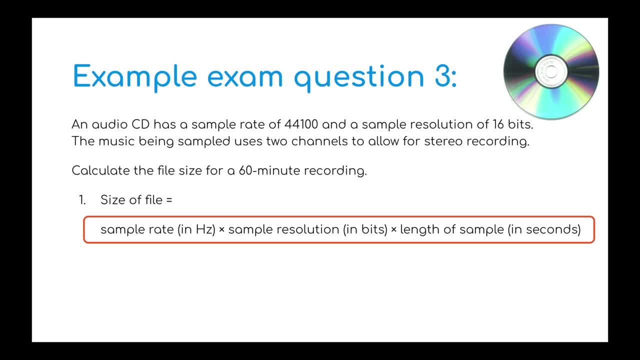 we've got 60 minutes of sampled recording, So let's have a look at this. The size of the sample would be 44,100.. It would be 44,100 times 16, times 60, times 60 again because, remember, we're working in.